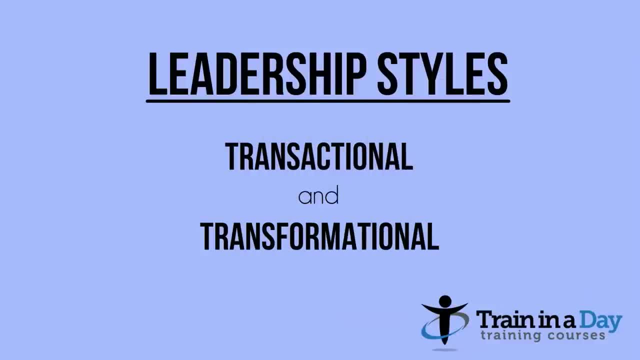 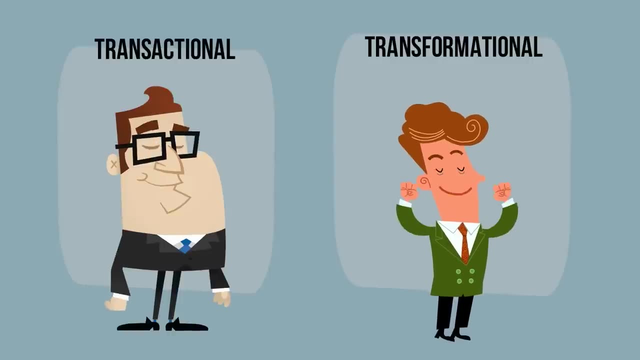 As an introduction, here are two common styles of leadership. One is called transactional and the other transformational. Once you've read through these two types, you'll be able to take a quick assessment in order to determine your own current leadership style, Whilst transactional leaders would. 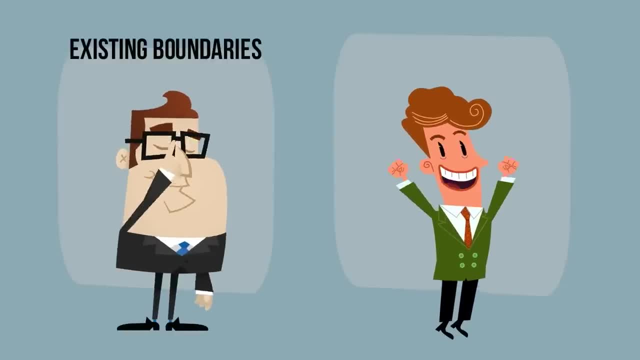 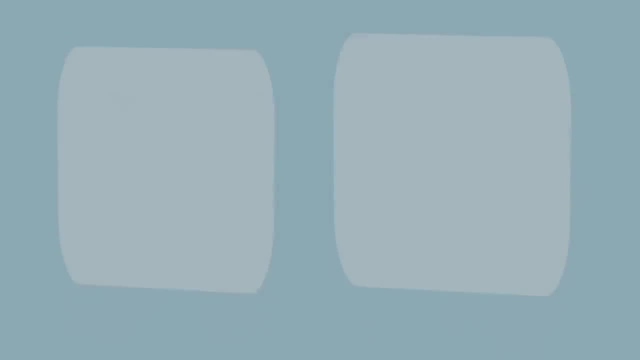 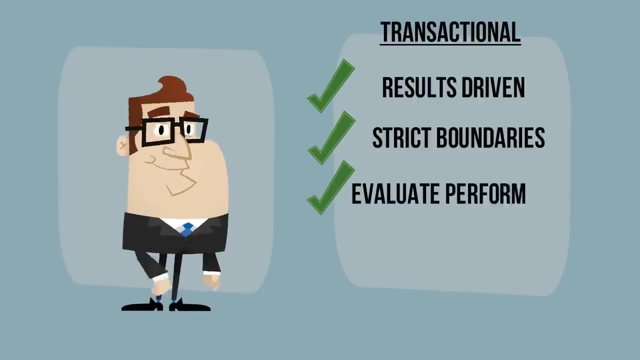 usually work within boundaries and have set established outcomes. a transformational approach is more future conscious and dynamic Transactional leadership. If you are a transactional leader, you'll be task and results driven, whilst adhering to strict organizational boundaries. Additionally, you'd be motivated to reward people and evaluate performance regularly. You'll be 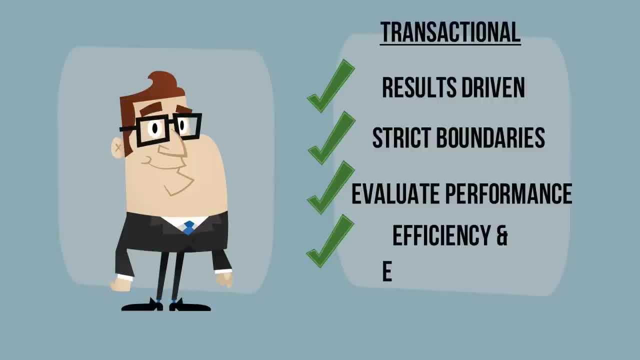 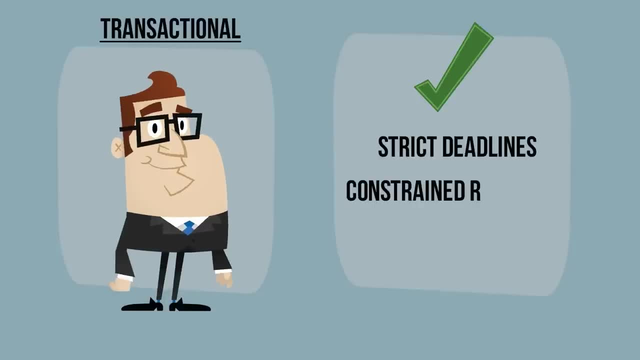 focused on ensuring activities are completed efficiently and effectively. This style of leadership can become especially useful when dealing with strict deadlines or are constrained with resources. It maintains group dynamics whilst evaluating how each team member or employee performs that given task. Transformational leadership: If you're a 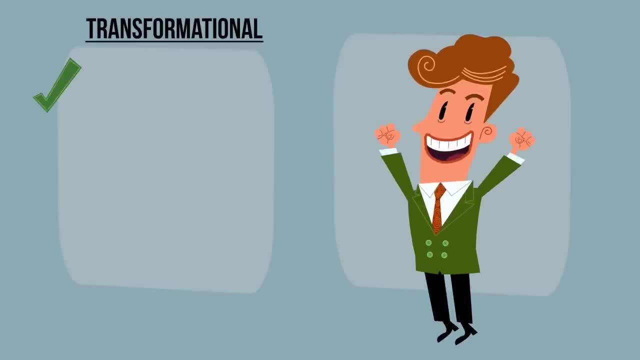 transformational leader, you'll focus on engaging and enthusing employees, Making sure they understand how their work will help deliver your vision within the company and the values of the organization. As a transformational leader, you'll lead by example whilst inspiring your team to drive change and achieve a common 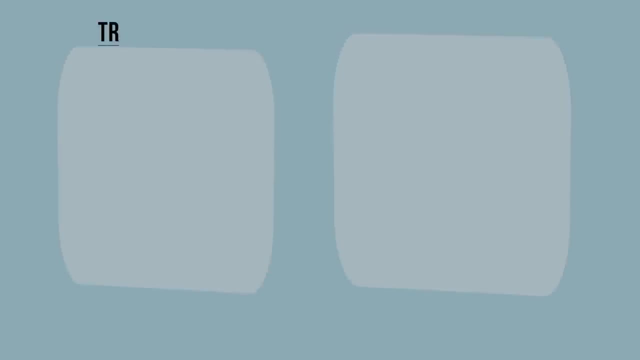 goal. There are important differences between transactional and transformational leaders. There are important differences between transactional and transformational leaders. A transactional leader will understand how rewarding someone will result in more effort being made, whilst a transformational leader will motivate their staff in order to get the 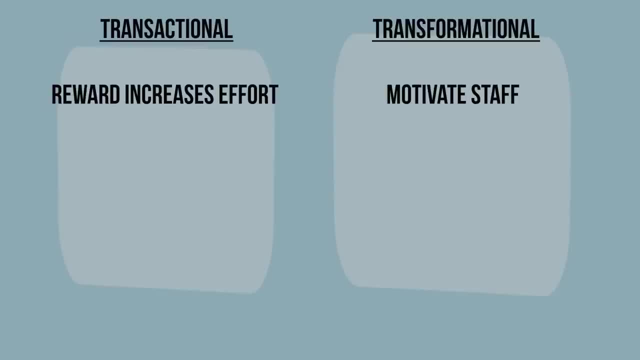 best out of them without having to constantly reward. Transactional leadership is more reactive to present concerns, whilst a transformational leader is more hands-on and, by doing this, creates higher expectations in their workers. A transactional leader will use methods such as carrot and stick motivation in order to control workers, as opposed to transformational leaders.